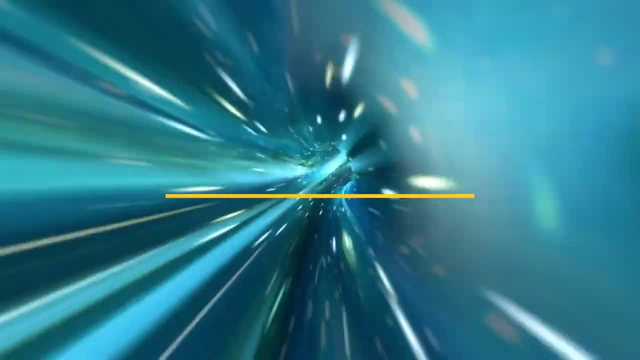 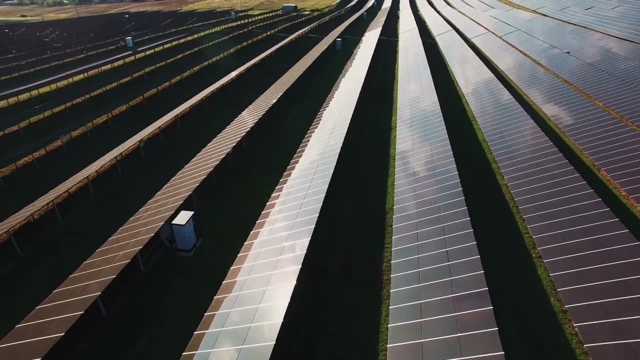 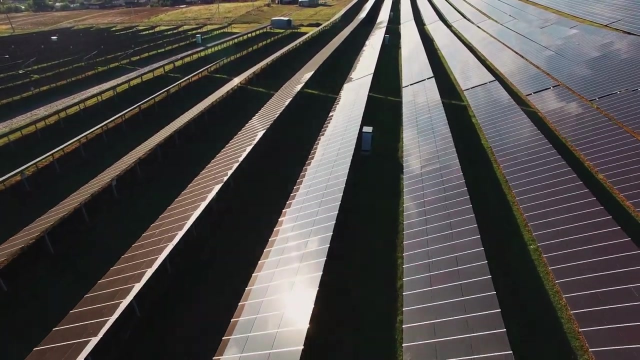 7 Types of Renewable Energy: 1. Solar. Solar energy is derived by capturing radiant energy from sunlight and converting it into heat, electricity or hot water. Photovoltaic PV systems can convert direct sunlight into electricity through the use of solar cells. Benefits: 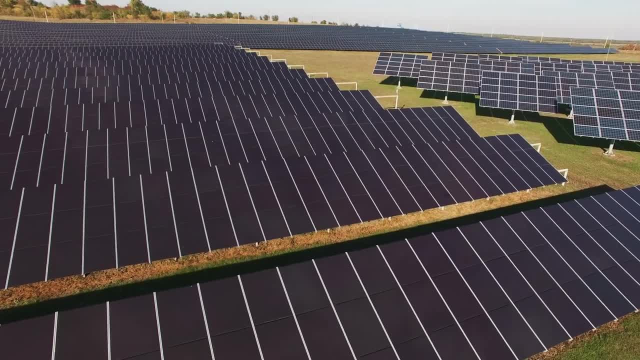 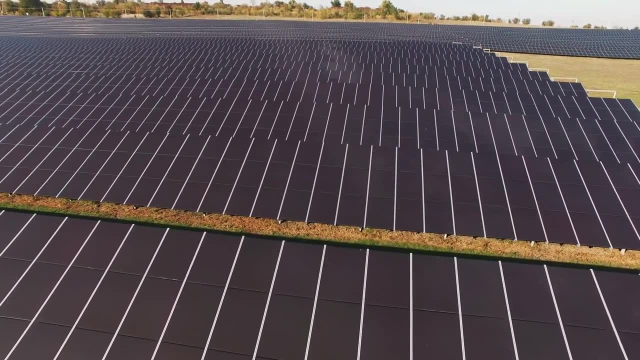 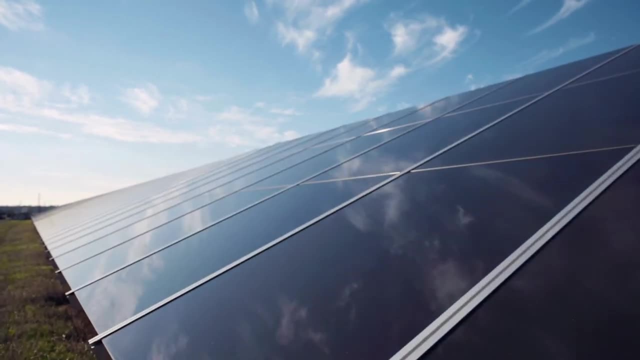 One of the benefits of solar energy is that sunlight is functionally endless With the technology to harvest it. there is a limitless supply of solar energy, meaning it could render fossil fuels obsolete. Relying on solar energy rather than fossil fuels also helps us improve public health and environmental conditions In the long term. 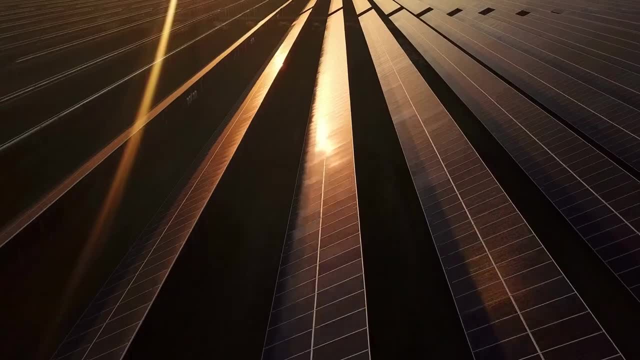 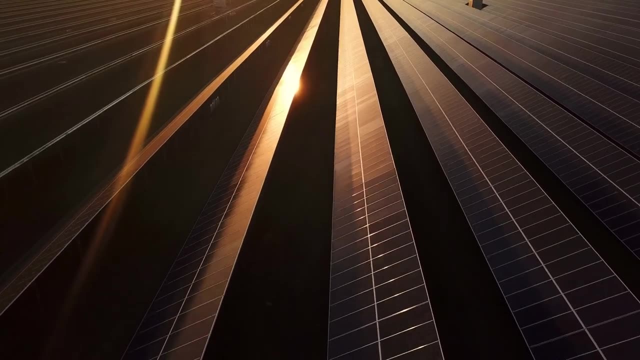 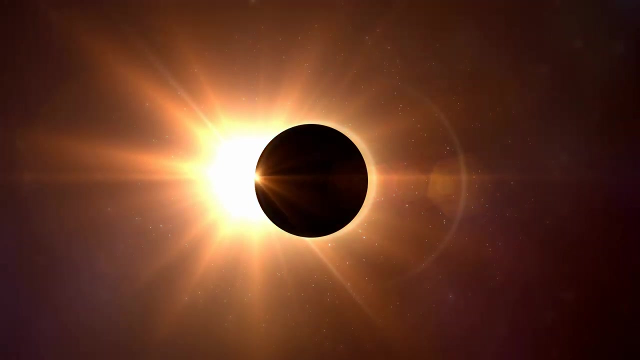 solar energy could also eliminate energy costs and, in the short term, reduce your energy bills. Many federal, local, state and federal governments also incentivize the investment in solar energy by providing rebates or tax credits- Current Limits. Although solar energy will save you money in the long run, it tends to be a significant 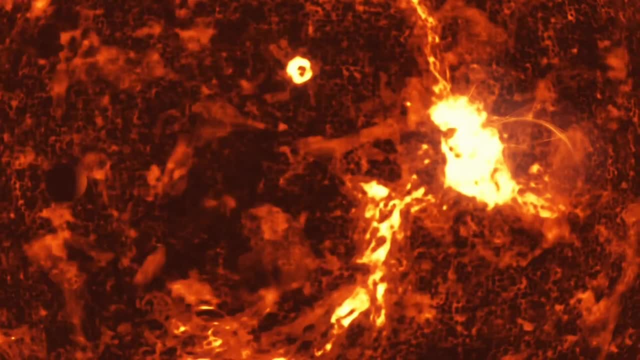 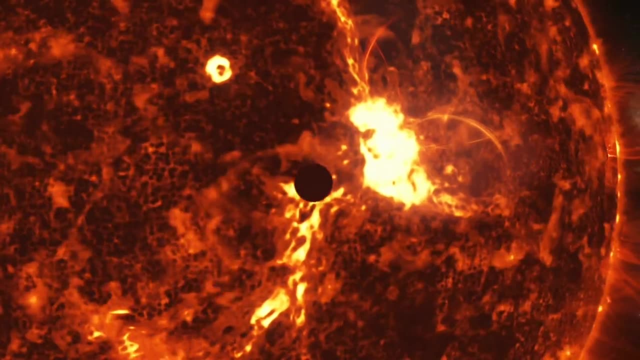 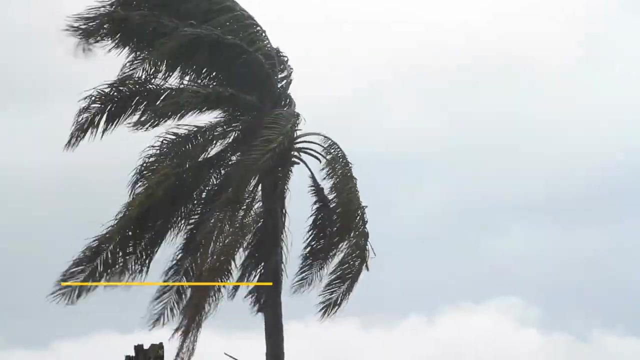 upfront cost and is an unrealistic expenses for most households. For personal homes, homeowners also need to have the ample sunlight and space to arrange their solar panels, which limits who can realistically adopt this technology at the individual level. 2. Wind- Wind farms capture the energy of wind flow by using turbines and converting it into electricity. 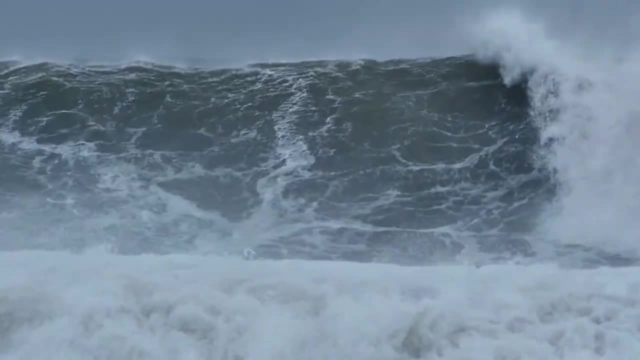 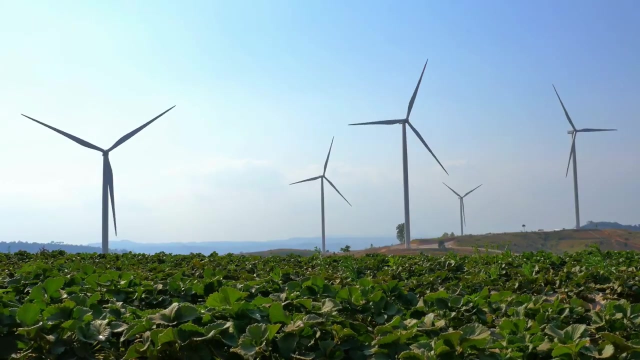 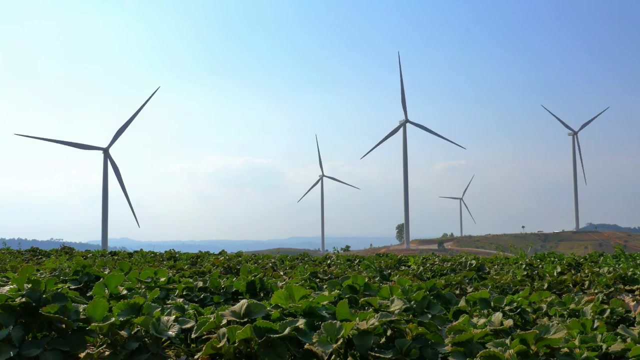 There are several forms of wind energy, Several forms of systems used to convert wind energy, and each vary Commercial-grade wind power generating systems can power many different organizations, while single wind turbines are used to help supplement pre-existing energy organizations. Another form is utility scale wind farms, which are purchased by contractor wholesale. 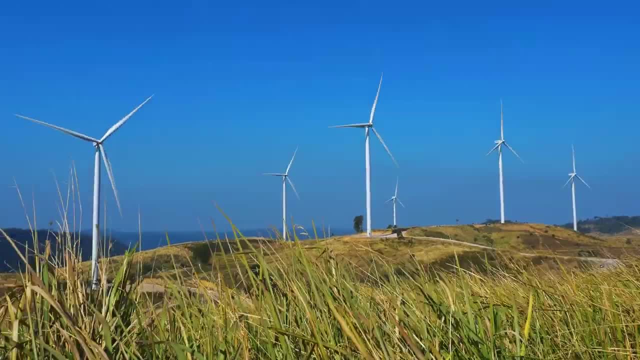 Technically, wind energy is a form of solar energy. The phenomenon we call wind is caused by the differences in temperature in the atmosphere combined with the rotation of Hearth and the Geography of Earth Wind causes. the reactor-based machines take up diese case of radiation and temperature. 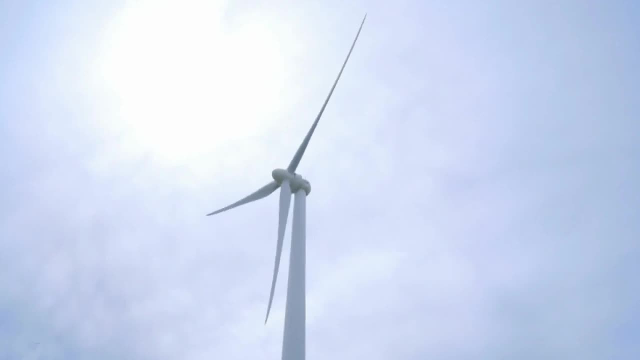 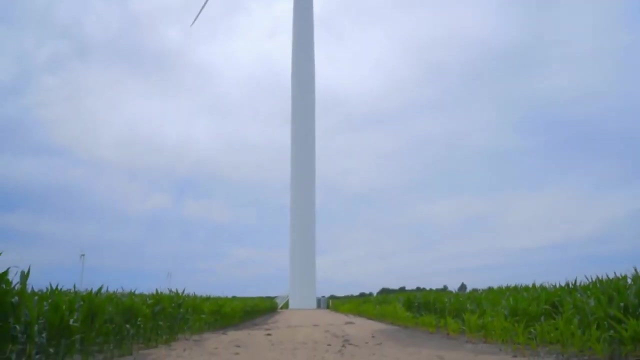 of earth and the geography of the planet benefits. wind energy is a clean energy source, which means that it doesn't pollute the air. like other forms of energy, wind energy doesn't produce carbon dioxide or release any harmful products that can cause environmental degradation or negatively affect human health, like smog, acid rain or other heat trapping gases. two: investment in wind energy. 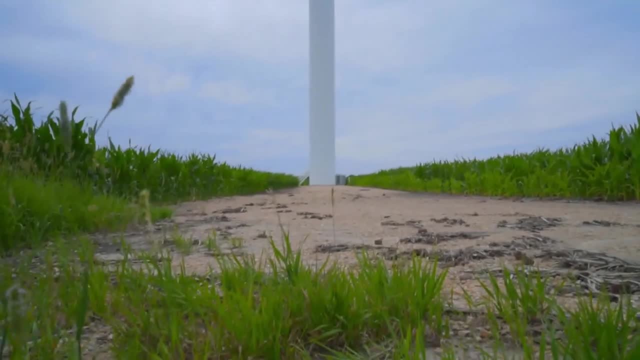 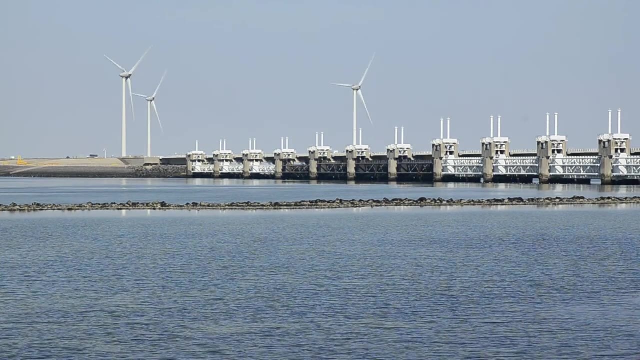 technology can also open up new avenues for jobs and job training, as the turbines on farms need to be serviced and maintained to keep running current limitations. since wind farms tend to be built in rural or remote areas, they are usually far from bustling cities where the electricity is. 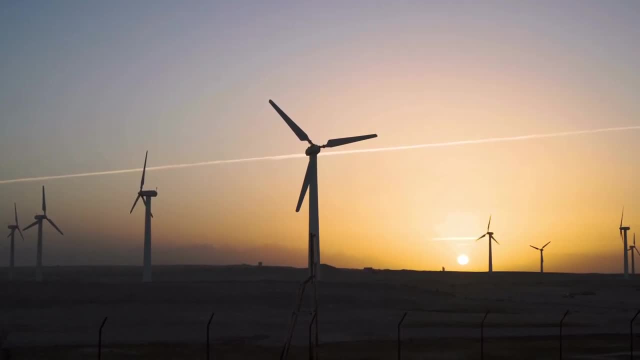 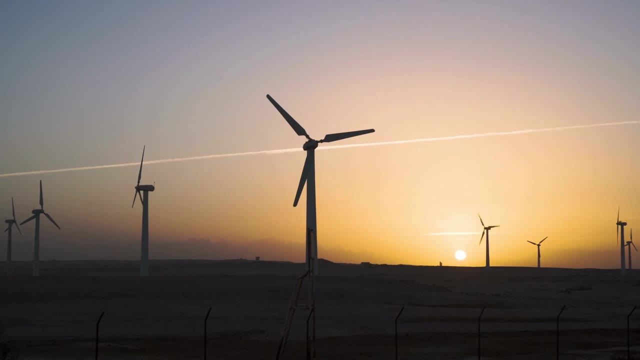 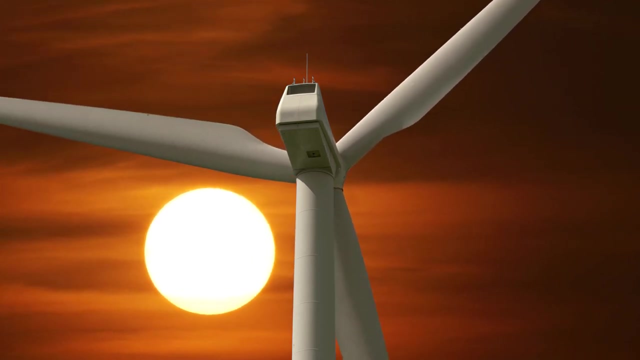 needed most wind energy must be transported via transition lines, leading to higher costs. although wind turbines produce very little pollution, some cities oppose them since they dominate skylines and generate noise. wind turbines also threaten local wildlife, like birds, which are sometimes killed by striking the arms of the turd. wind turbines can also be used as a source of energy. 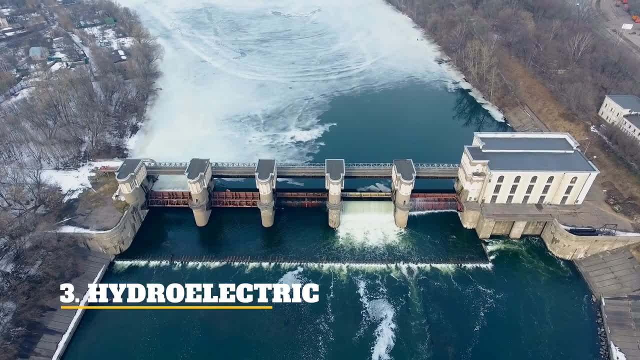 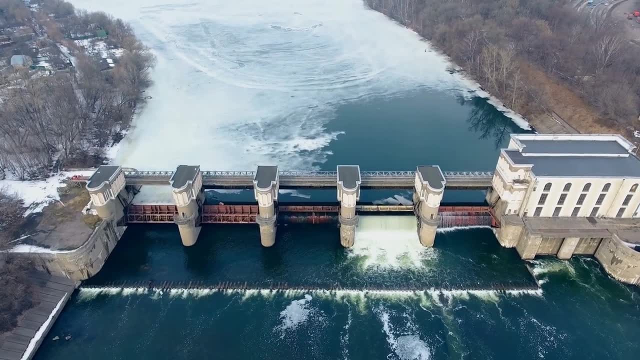 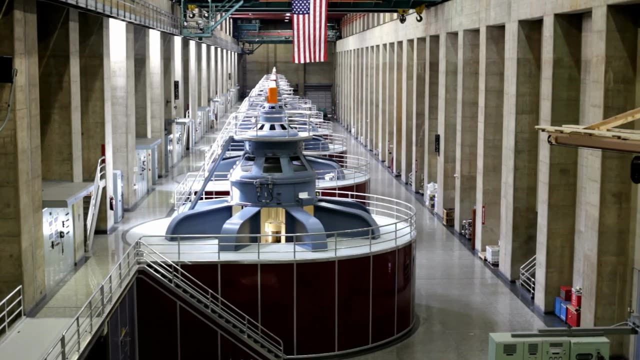 while flying. three hydroelectric dams are what people most associate when it comes to hydroelectric power. water flows through the dam's turbines to produce electricity, known as pumped storage hydropower. run of river hydropower uses a channel to funnel water through rather than powering it through a dam. benefits hydroelectric 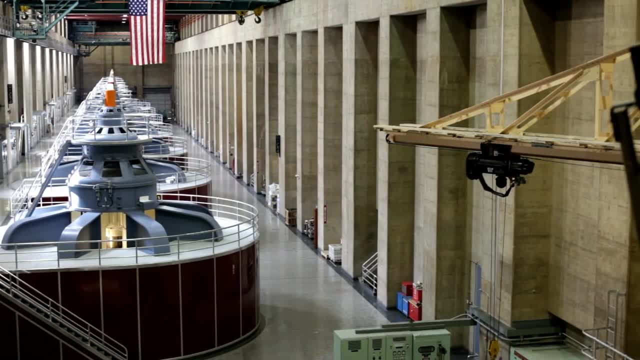 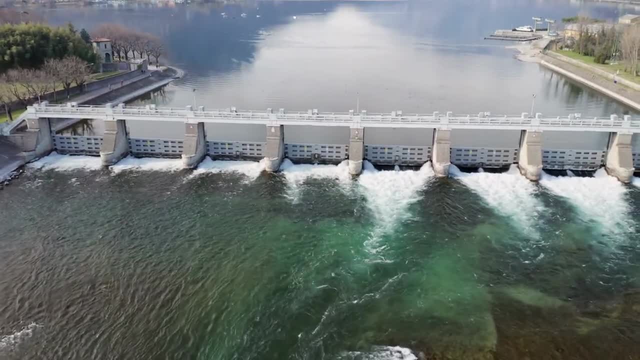 power is very versatile and can be generated using both large-scale projects like the hoover dam and small-scale projects like wind turbines. wind turbines can be used to generate electricity, projects like underwater turbines and lower dams on small rivers and streams. hydroelectric power does not generate pollution and therefore is a much more environmentally friendly energy option. 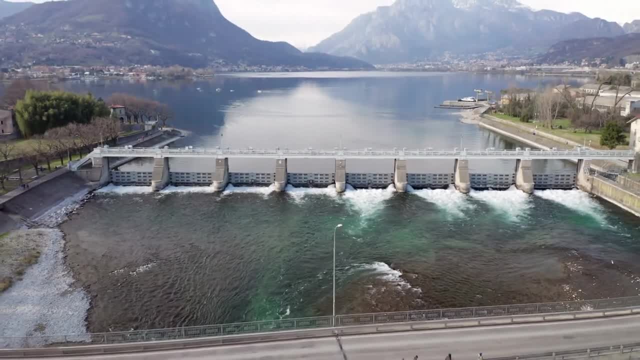 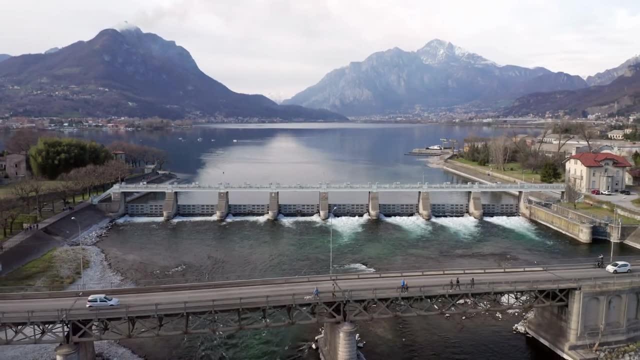 for our environment. current limitations: most us hydroelectricity facilities use more energy than they are able to produce for consumption. the storage systems may need to use fossil fuel to pump water free. although hydroelectric power does not pollute the air, it disrupts waterways and 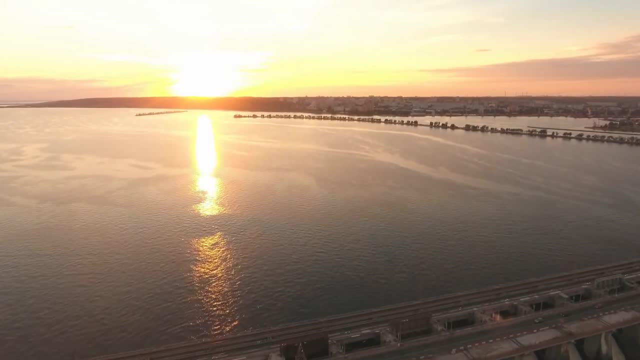 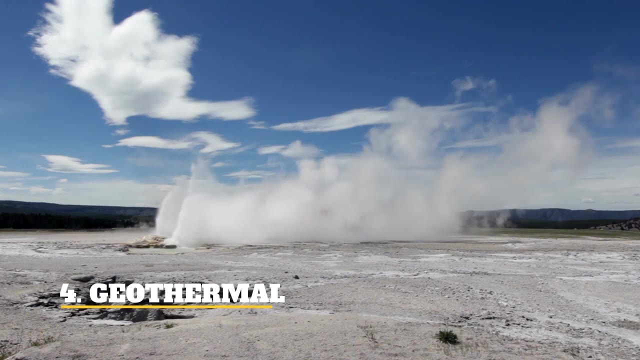 negatively affects the animals that live in them and the environment they live in, can be used to generate electricity for the environment, they will have to change water levels, currents and migration paths for many fish and other freshwater ecosystems for geothermal. geothermal heat is heat that is trapped beneath the earth's crust from the formation of the earth. 4.5 billion years ago and from radioactive decay. sometimes large amounts of this heat escapes naturally but all at once, resulting in familiar occurrences such as volcanic eruptions and geysers. this heat can be captured and used to produce geothermal energy to decrease the water. 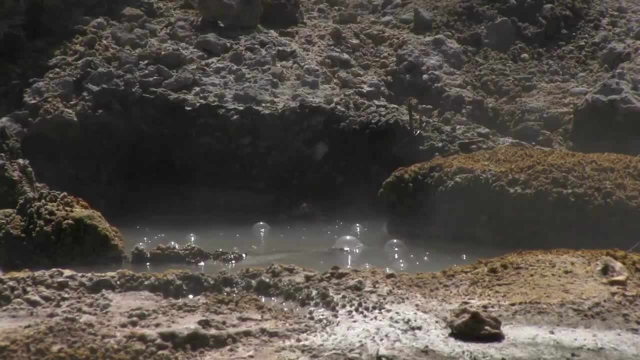 energy by using steam that comes from the heated water pumping below the surface, which then rises to the top and can be used to operate a turbine Benefits. Geothermal energy is not as common as other types of renewable energy sources, but it has a significant potential for energy supply, Since it can be built underground. 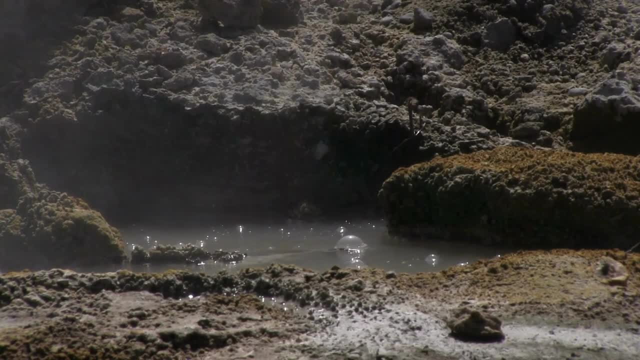 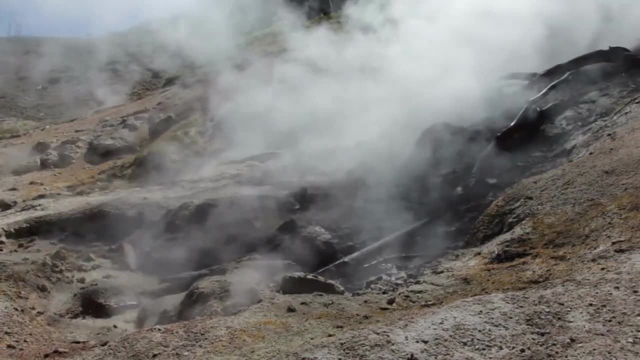 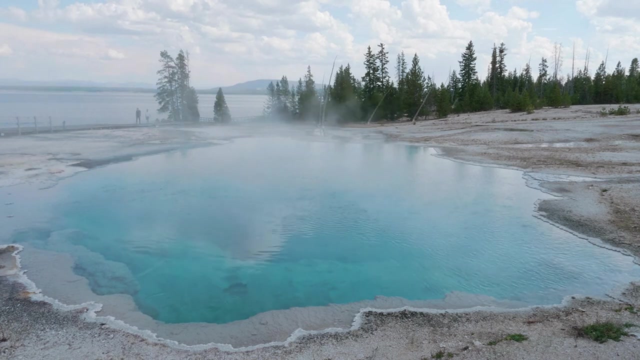 it leaves very little footprint on land. Geothermal energy is naturally replenished and therefore does not run a risk of depleting on a human timescale. Current limitations: Cost- plays a major factor when it comes to disadvantages of geothermal energy. Not only is it costly to build the infrastructure, but another major concern- 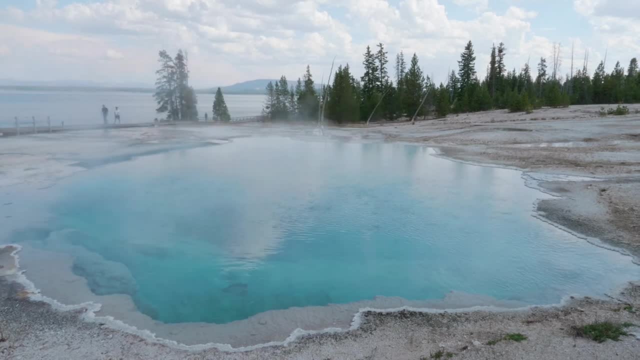 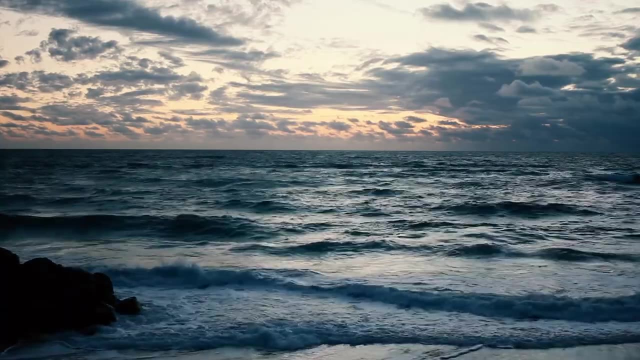 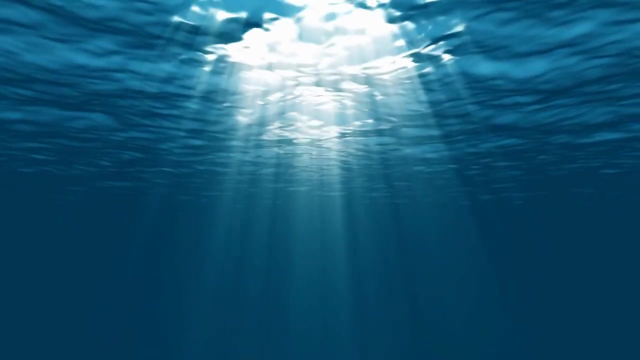 is its vulnerability to earthquakes in certain regions of the world. 5. Ocean: The ocean can produce two types of energy: thermal and mechanical. Ocean thermal energy relies on warm water surface temperatures to generate energy through a variety of different systems. Ocean mechanical: 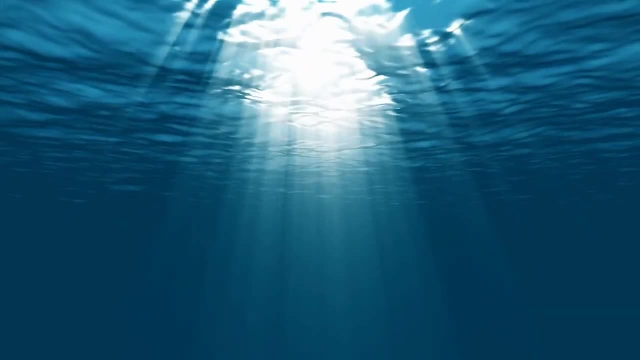 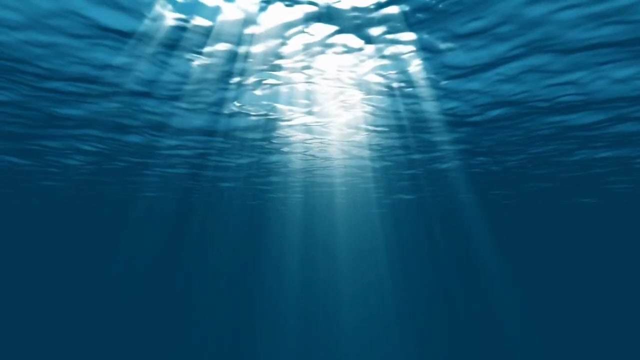 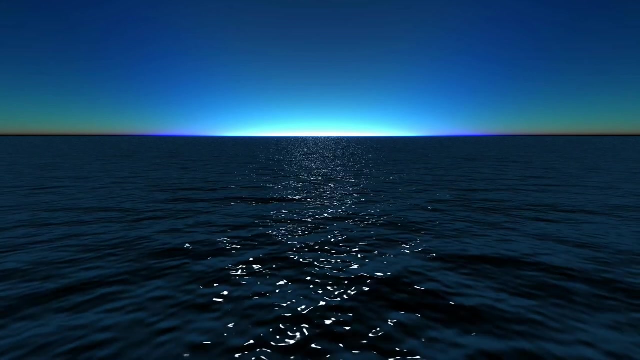 energy uses the ebbs and flows of the tides to generate energy, which is created by the earth's rotation and gravity from the moon Benefits. Unlike other forms of renewable energy, wave energy is predictable and it's easy to estimate the amount of energy that will be produced, Instead of relying on varying factors such as. 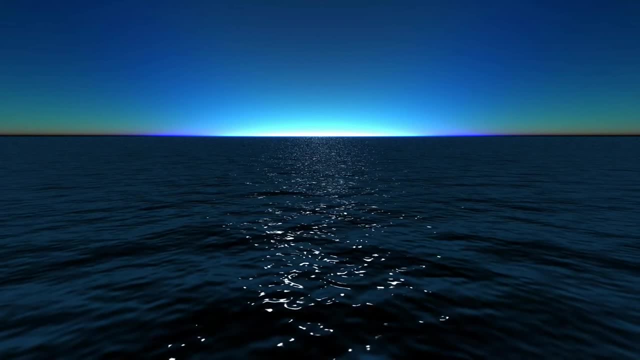 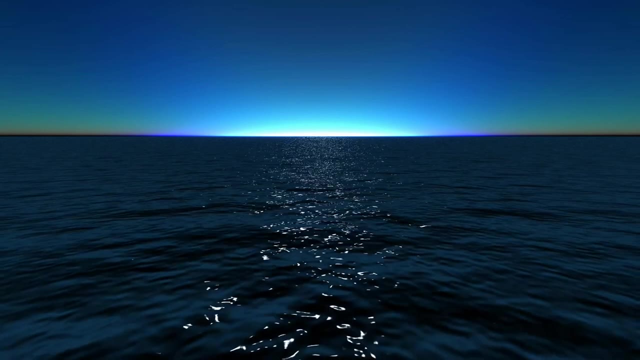 sun and wind, wave energy is much more consistent. This type of renewable energy is also abundant. the most populated cities tend to be near oceans and harbors, making it easier to harness this energy for the local population. The potential of wave energy is an astounding, as yet untapped. 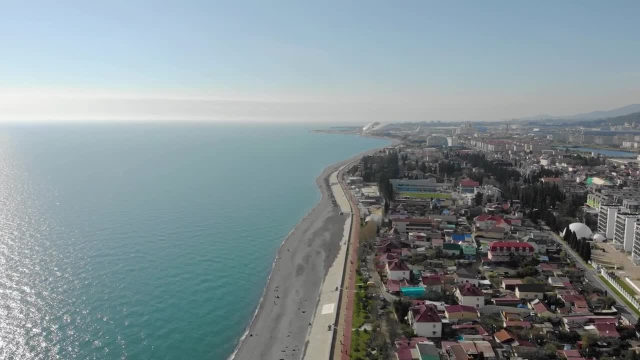 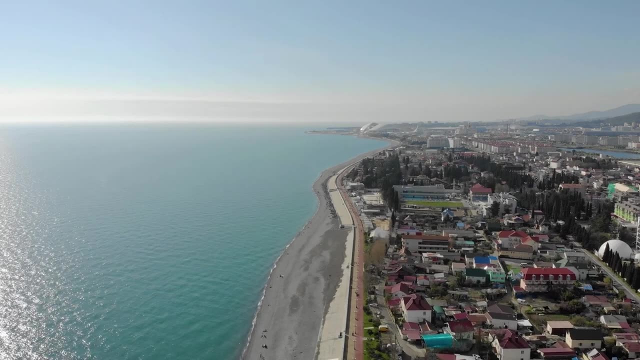 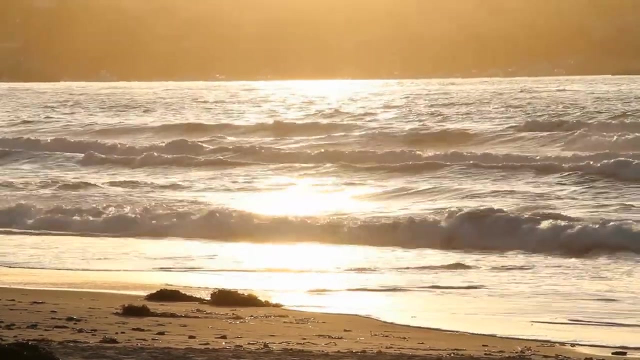 energy resource with an estimated ability to produce 2,640 terawatt hours per year. Just 1 terawatt hour per year of energy can power around 93,850 average US homes with power annually, or about twice than the number of homes that currently exist in the US at present. 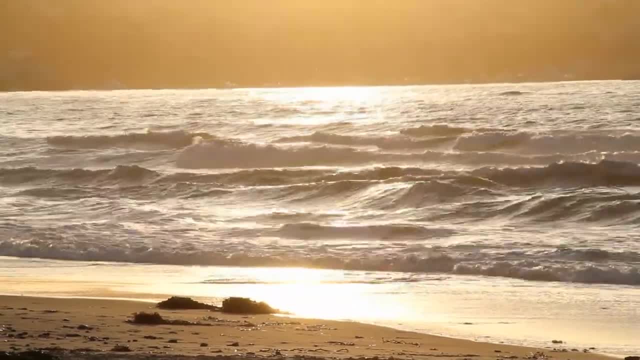 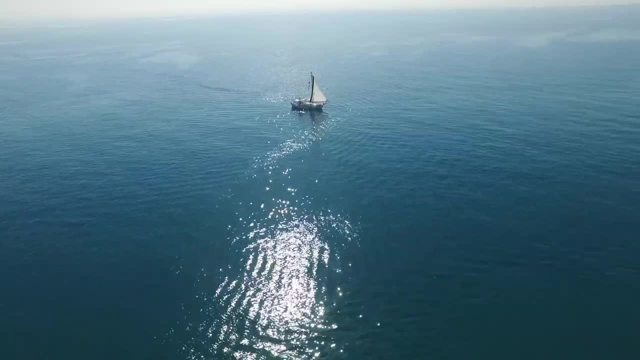 Current limitations. Those who live near the ocean definitely benefit from wave energy, but those who live in landlocked states won't have ready access to this energy. Another disadvantage to ocean energy is that it can disturb the ocean's many delicate ecosystems, Although it is a very clean 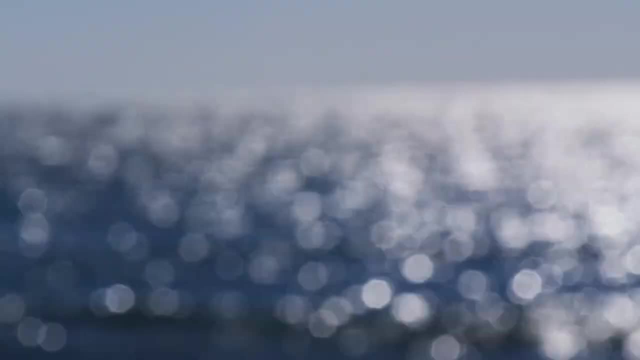 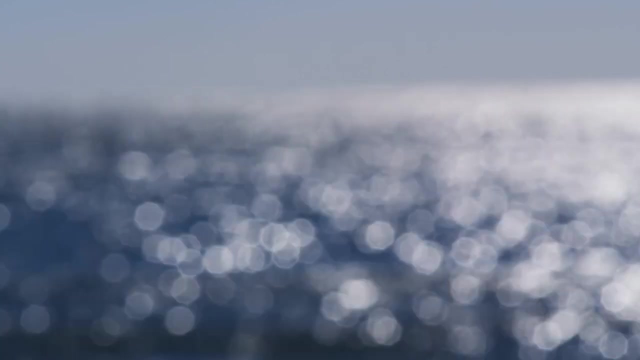 source of energy. large machinery needs to be built nearby to help capture this form energy, which can cause disruptions to the ocean floor and the sea life that habitats it. Another factor to consider is weather. when rough weather occurs, it changes the consistency of the 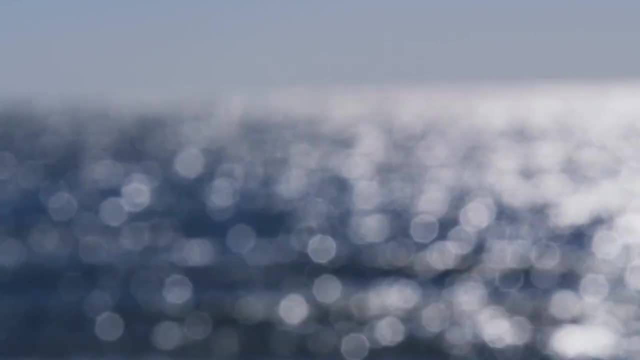 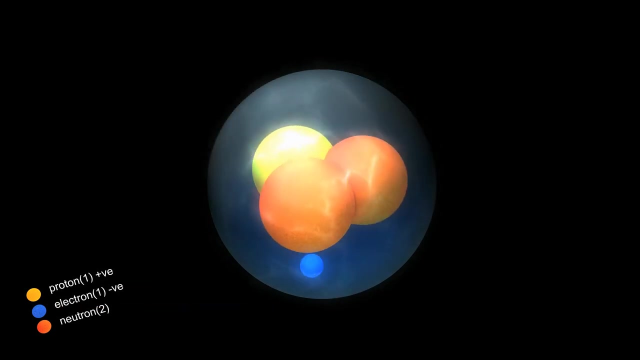 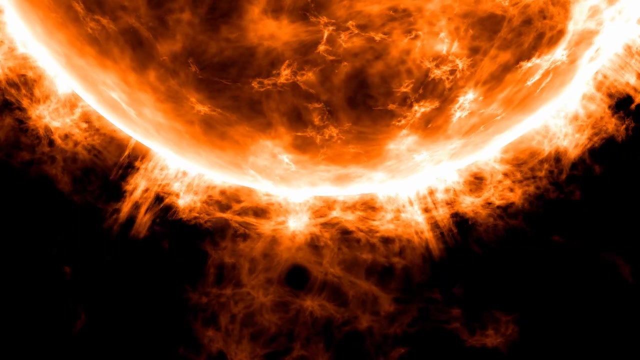 waves, thus producing lower energy output when compared to normal waves without stormy weather. 6. Hydrogen: Hydrogen needs to be combined with other elements, such as oxygen, to make water, as it does not occur naturally as a gas on its own When hydrogen is separated from another element.